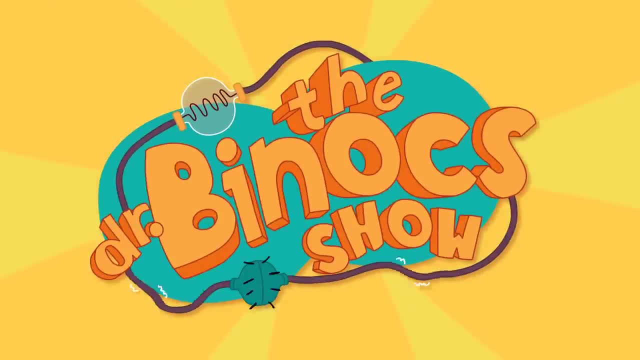 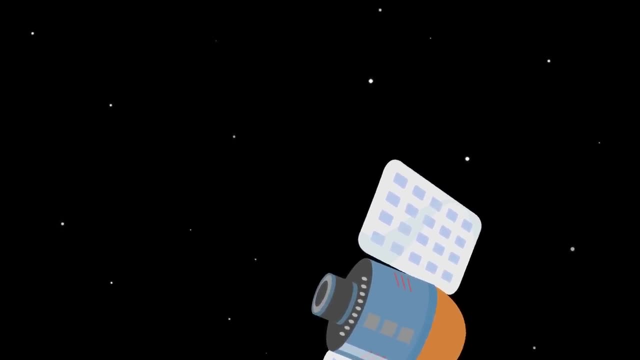 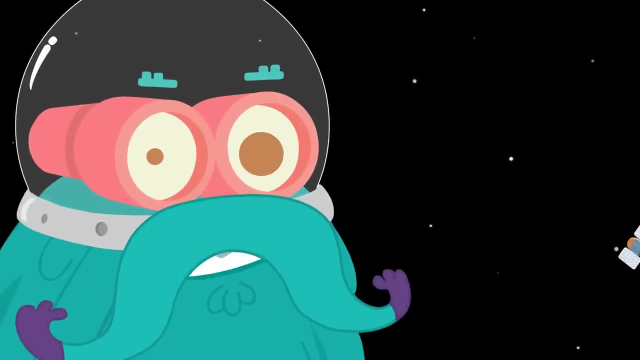 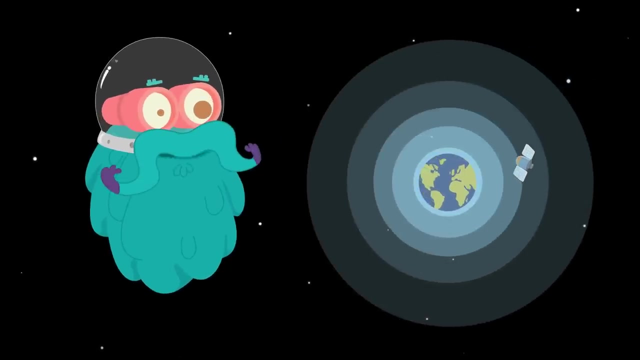 Hey, everyone guess where I am? Well, don't think so hard. I am in space. Do you see that blue ball? Well, that's where you are. That's the Earth. But hey, what are these? They are the layers of atmosphere. 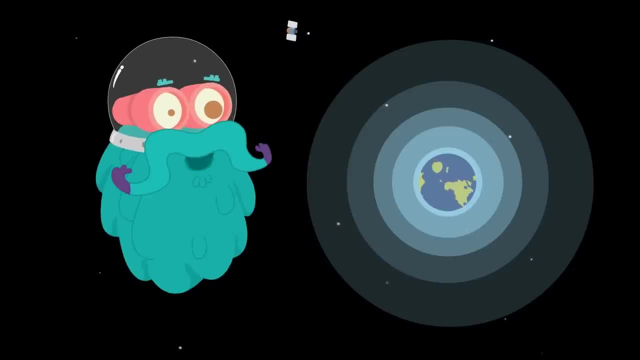 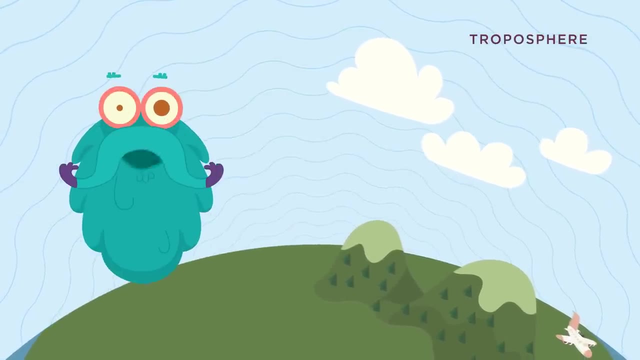 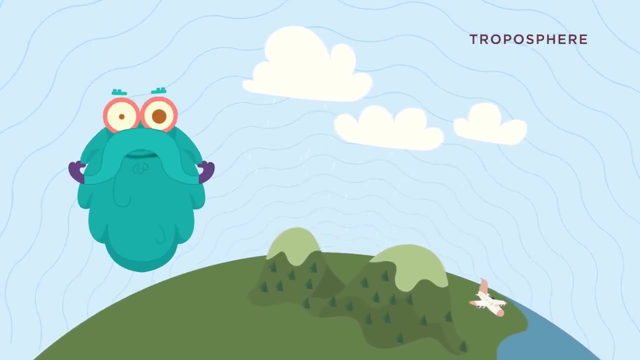 So let's learn about the layers of atmosphere today. Zoom in. This is the Troposphere. This layer is where the weather occurs. This is the lowest atmospheric layer and begins at the surface of the Earth and extends out to about 4 to 10 miles. 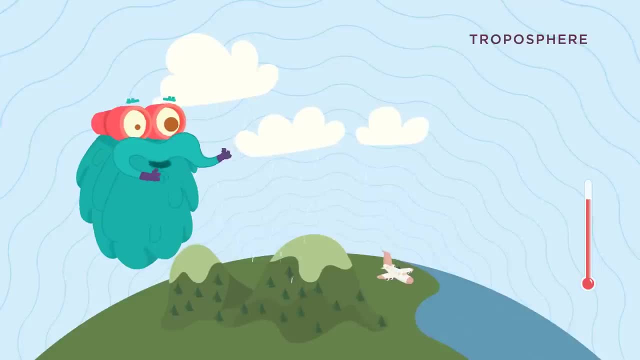 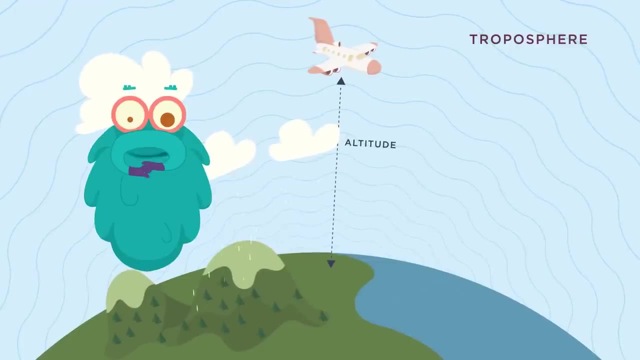 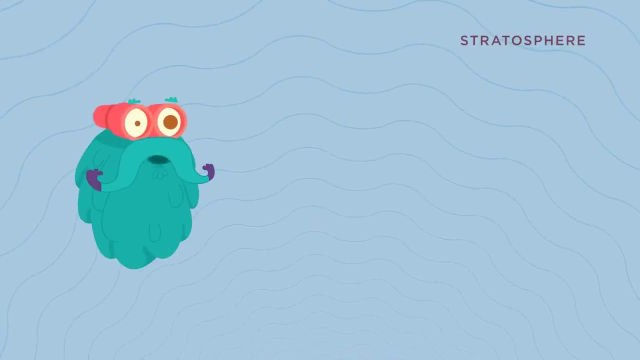 The temperature of the Troposphere decreases with increase in altitude. Just so that you know, altitude is the height of an object or point in relation to the ground level. Now we are in the Stratosphere, second lowest layer of Earth's atmosphere. 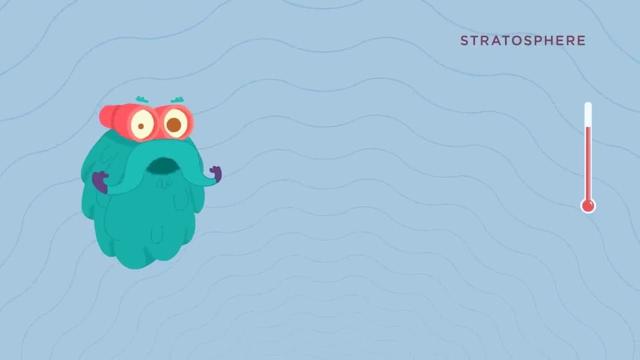 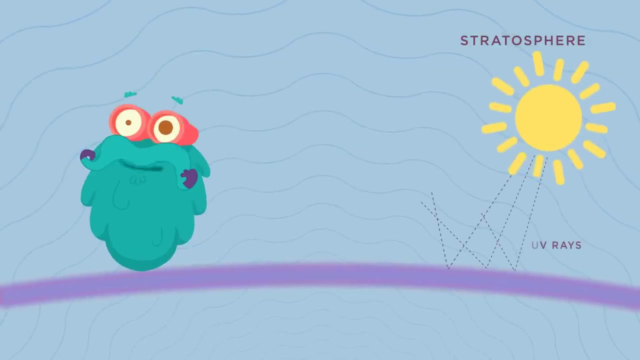 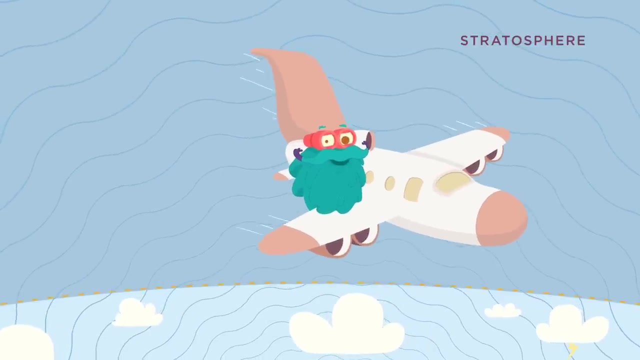 Here, the temperature rises with the rise in altitude. You will also find the Ozone layer here, which helps absorb harmful UV rays from the Sun. This is the layer where you will find aeroplanes flying around, As the Stratosphere is free of all weather disturbances. 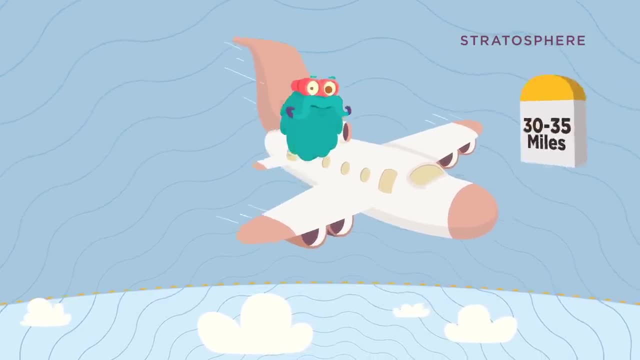 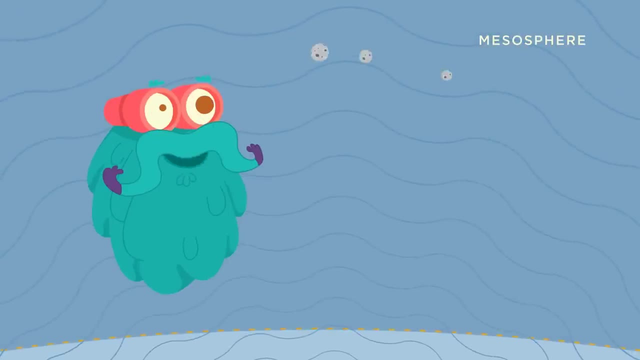 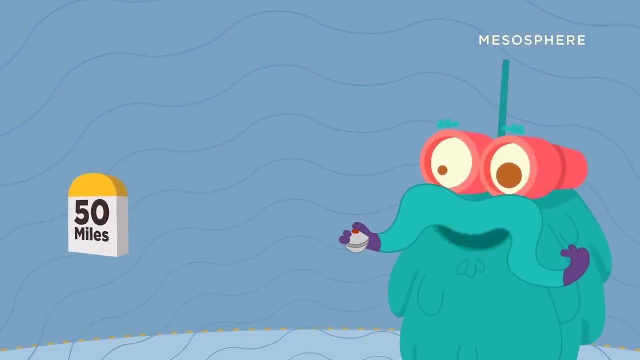 The Stratosphere extends to about 30 to 35 miles above the Earth's surface. This is the Mesosphere where most meteors burn upon entry. The Mesosphere stretches up till 50 miles from the Earth's surface. The Thermosphere is next. 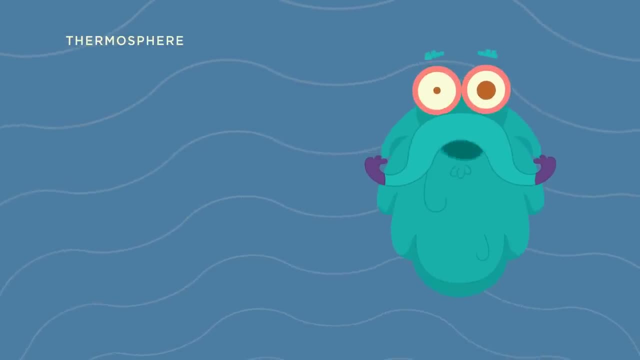 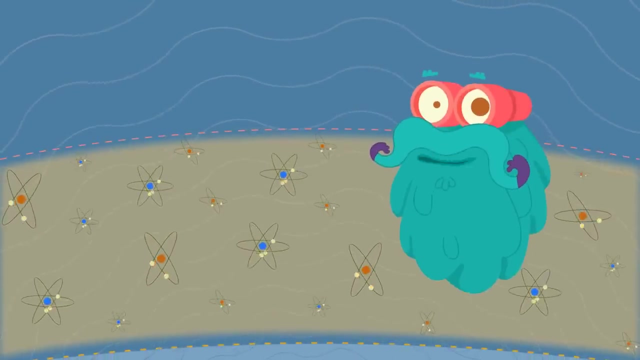 And the air is very thin. here, Temperatures get extremely hot. in the Thermosphere It extends up to 400 miles from the Earth's surface. The lower part of this layer contains the Ionosphere. Many atoms are ionized in this layer and you will also find electrical charge here.